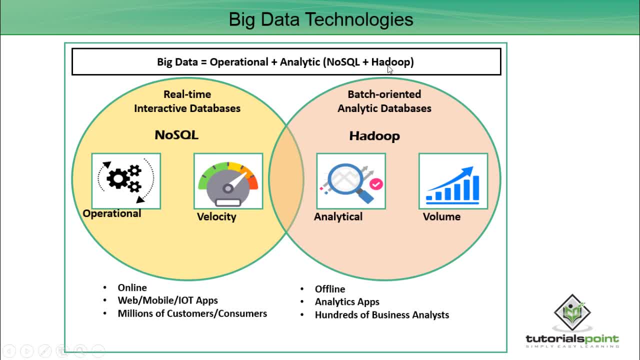 What about the operational efficiencies we are expecting and cost reductions we are expecting in the decision-making resulting for the better implementation? Everything can be obtained in under aiana also. Everything can be obtained and our business will succeed. 26对不能 about big data technologies. so there are various technologies in the market for for from different 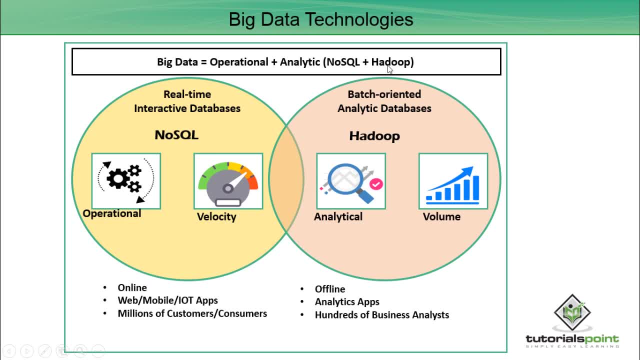 vendors, including our amazon. we are having ibm, microsoft, etc. to handle big data and basically there are two classes to handle big data. so what are the two classes? so, as we have explained, as we have discussed, that is the operational big data and analytical big data. so at first we are 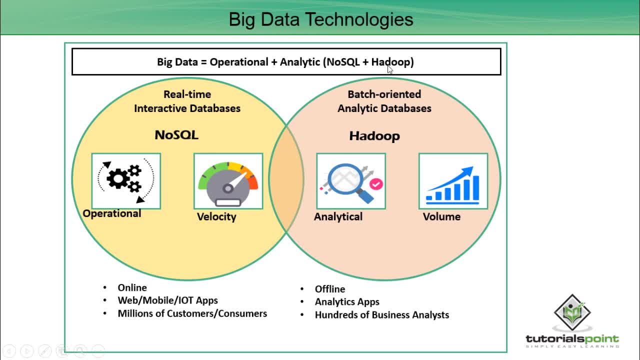 going for this operational big data which works on real-time interactive databases- no sql will be there and we will be having the huge velocity that means huge data will be produced- the rate of production of the data will be too huge- and which will be working online for the web, mobile and iot. 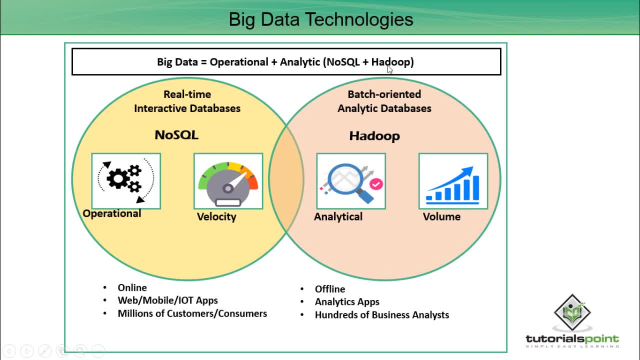 applications and millions of customers and consumers will be related with this operational big data. so this technology is actually the no sql database, like our mongodb, that provides operational compatibilities for the real-time applications and no sql basically will be there and we will be having the huge velocity. that means huge data will be. 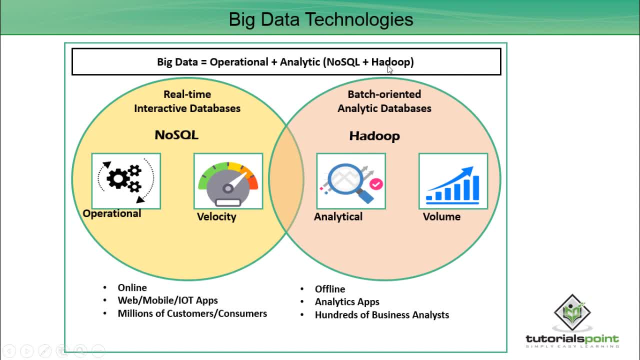 generated, and the big data systems are designed to take the advantage of new cloud computing architectures that have emerged over the past decade to allow massive computations to be run inexpensively and also efficiently. so that is one of the main advantage of this operational big data, and some no sql systems can provide insights into the pattern and the trends based on the real-time. 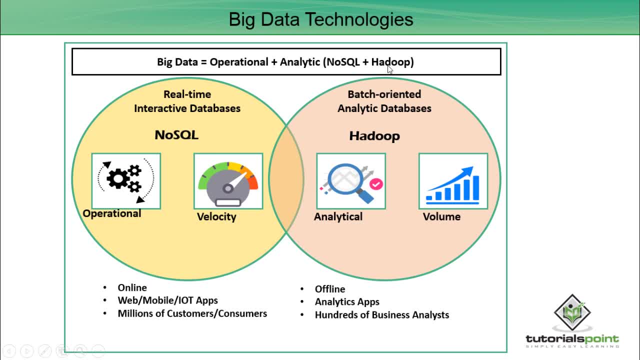 data with minimal data coding and without the need for data scientists and for also additional infrastructure so we can find out the respective pattern or we can provide some insights of the pattern in our data without having any additional expenses, without having any educational infrastructure and data scientists. now, what is the analytical big data? so analytical big data is actually the batch oriented.